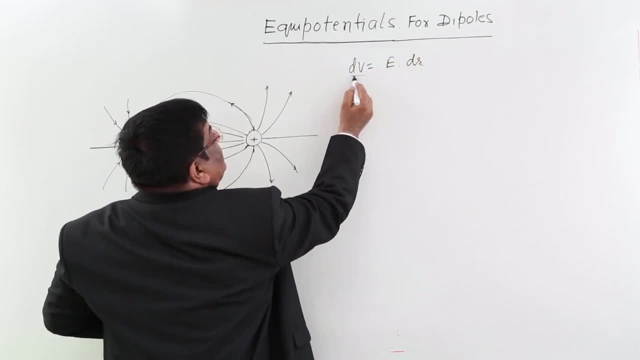 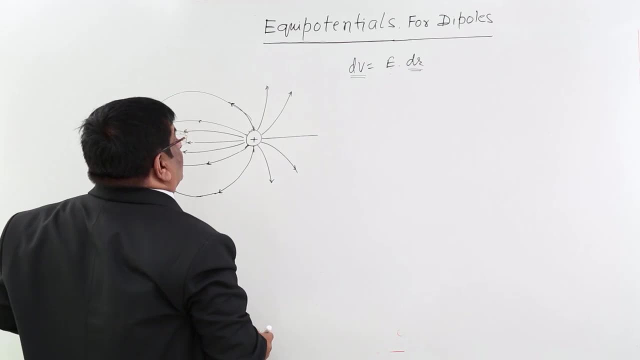 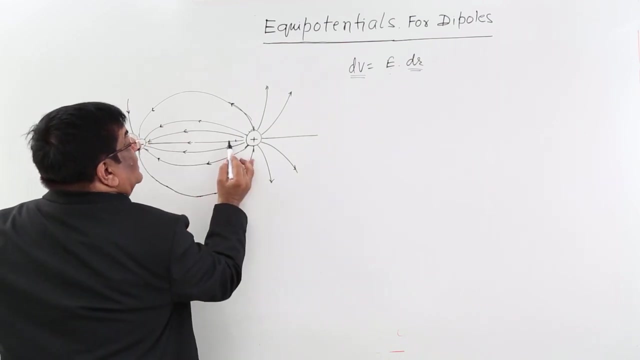 to E dr. If we take dv, electric field become weak, then dr has to become large. So here we get 5 volt. here we get, say, 10 volt, 10 volt, 5 volt, this much distance, Here we get 5 volt and here. 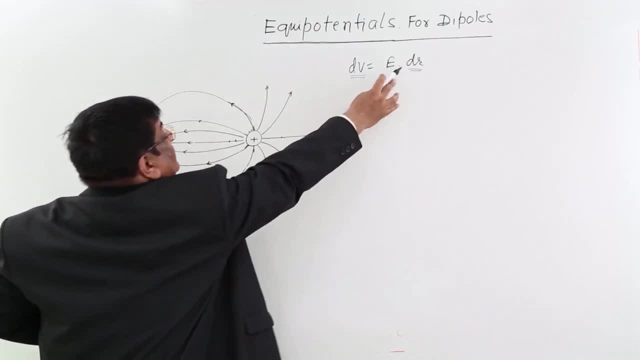 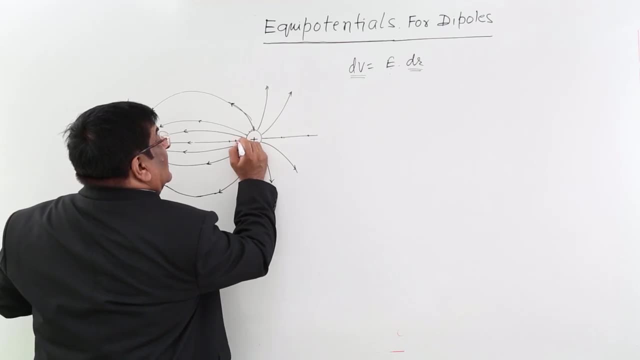 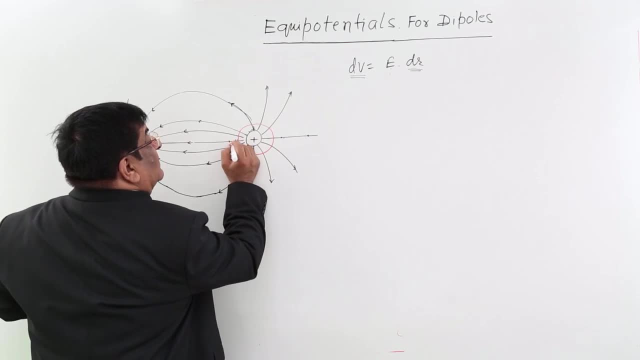 is equal to dv. so all these, molto is equal to dv. So dv, dv is equal to dv and this is equal to dv is equal to 0.. So dv, dv is equal to dv. So dv is equal to dv. and if you limit, 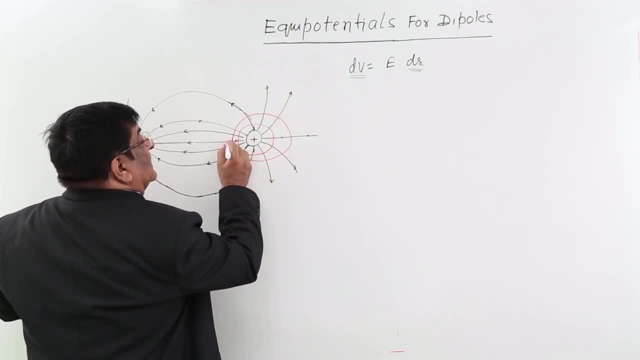 dv to per unit, then go to p cos k, dv plus in terms of e, доллар times, f and m cos q. by m See, dv is equal to eom角. it is equal toool four divided by k plus m plus q, into r plus e, n, d, p, c, ik, and it actually means: 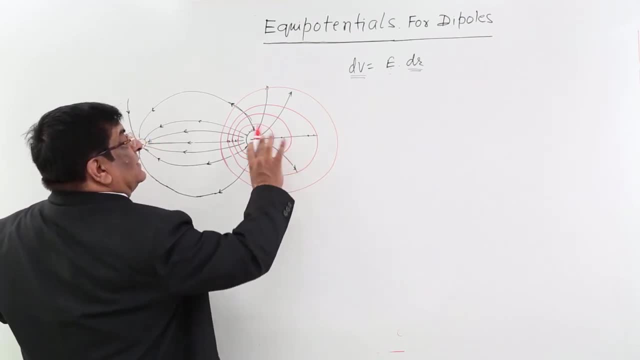 0.. Can this rooking terus on the c? ş? This is a big job to do. if we can writeero the re maybeскимine of r to riㅎЗ k. marriage is very close to this. Here it is a close distance and here it will be larger distance. 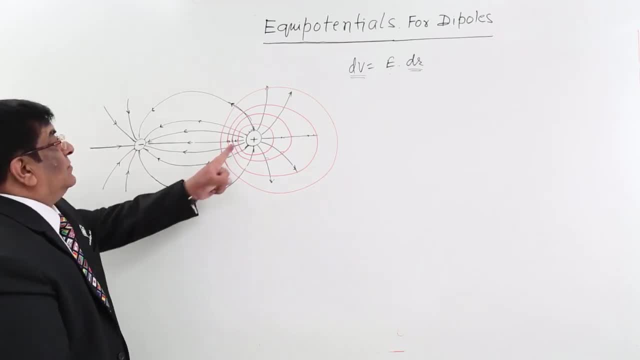 So it will be like this: Now we know that plus and minus at center, the potential is 0. If potential is 0 on equatorial line, we will find no equipotential there. or we can say there is an equipotential which is like this: and this equipotential has how much potential. 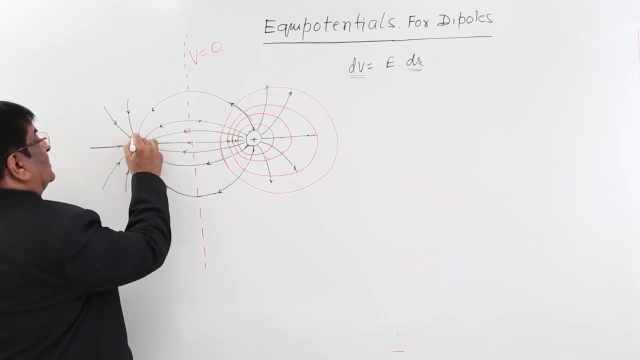 So here we get equipotentials this way: this 2,, 3,, 4, this is 2,, this is 3,, this is 4, the distance we go on increasing on this side like this. So these are the equipotentials. 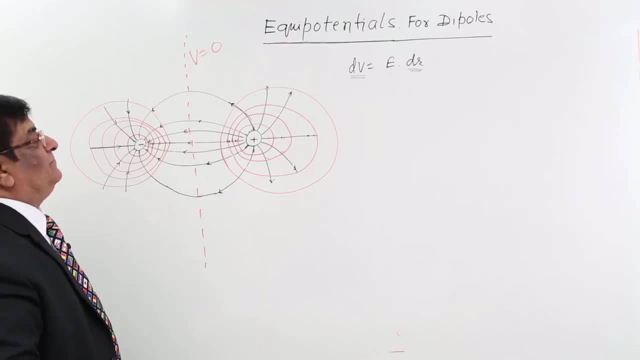 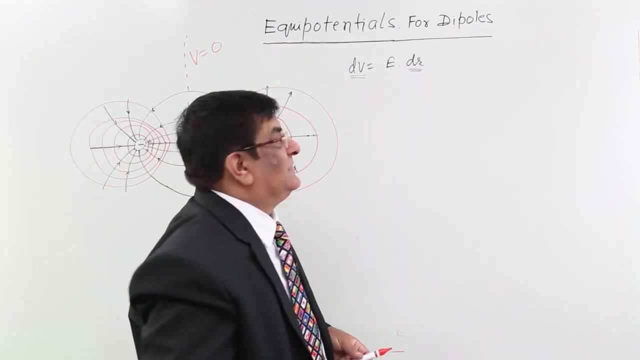 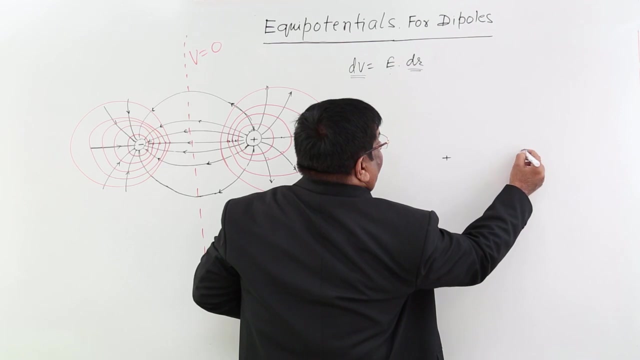 for plus and minus, 2 types of charges. Here they are closer, here they are going away because electric field is getting weak here and at centre. this is V is equal to 0. we can take it as a equipotential. Now if the two charges are similar charges like plus and plus, plus and plus from very 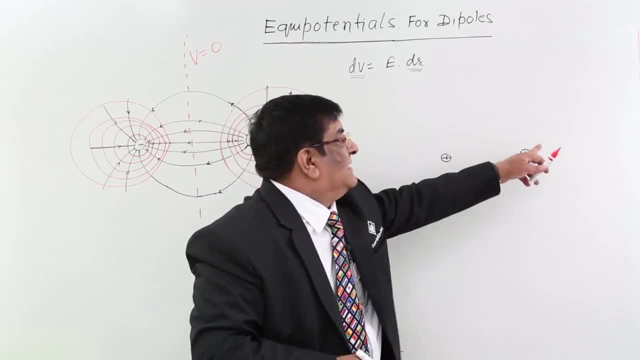 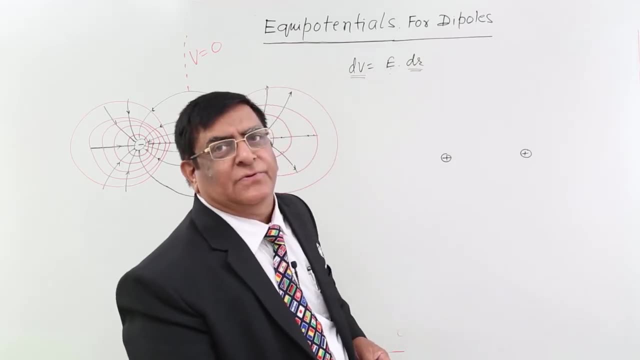 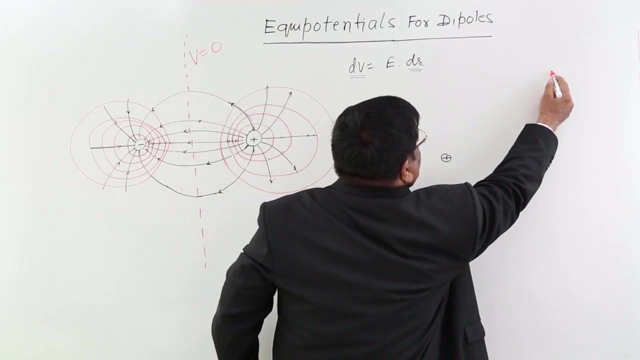 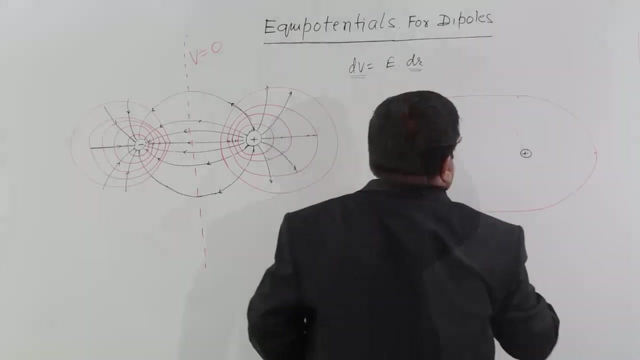 far away. when we say we see this as a system of two positive charges. they are very close, we are far away, so what type of potential? we get this distance, this distance, this distance or almost same from these two and we get a equipotential like this: 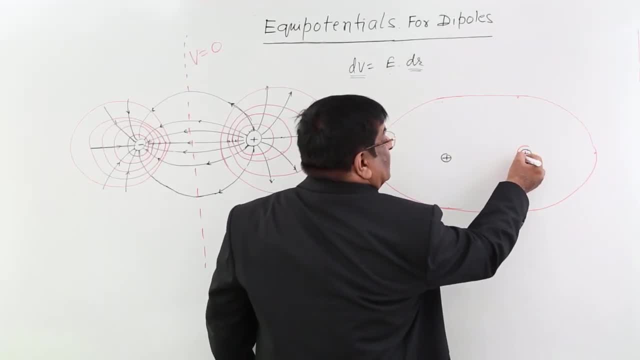 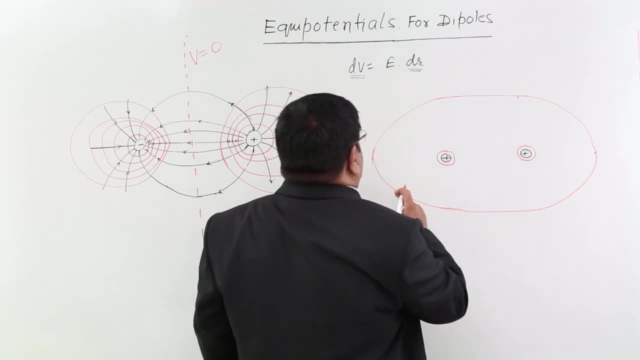 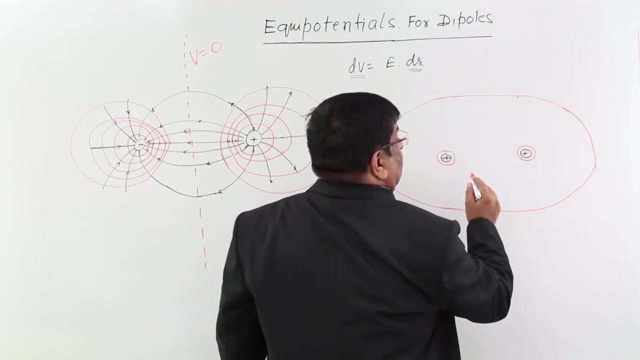 But as we come closer, very close to it, this is equipotential surface for this, and this is equipotential surface for this, and this is equipotential surface for the complete system. Now, how it has happened. so then, what will be the in between? see, in between, this will. 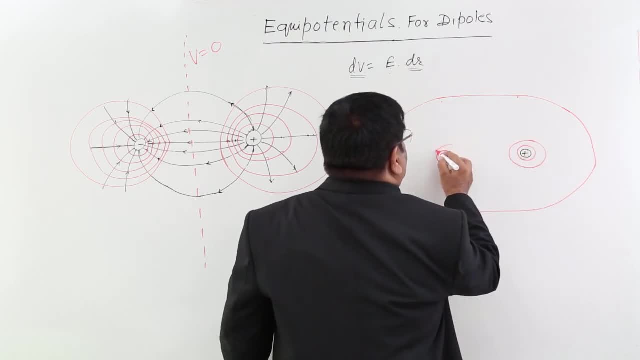 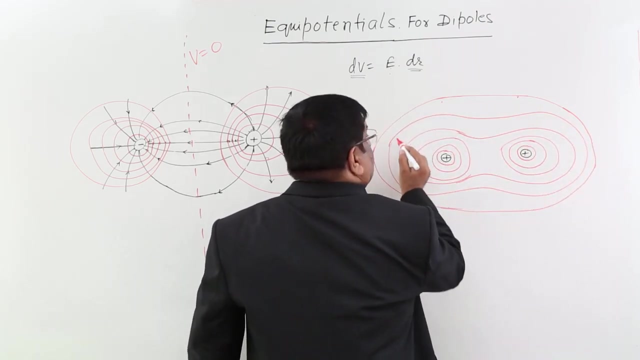 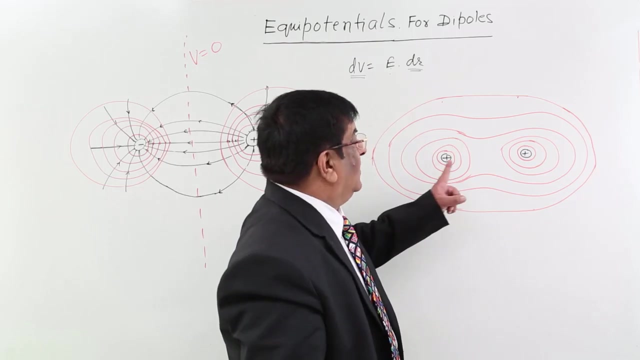 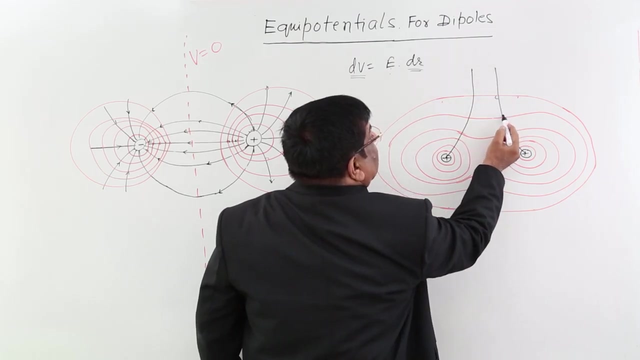 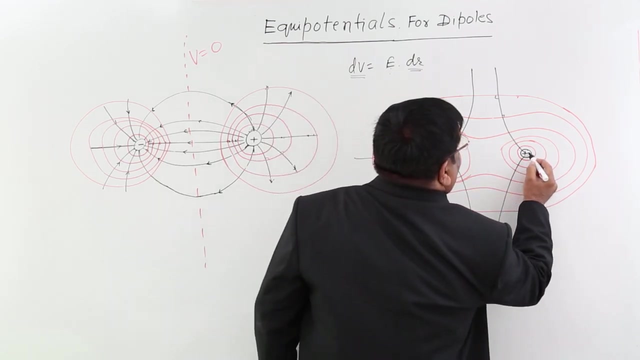 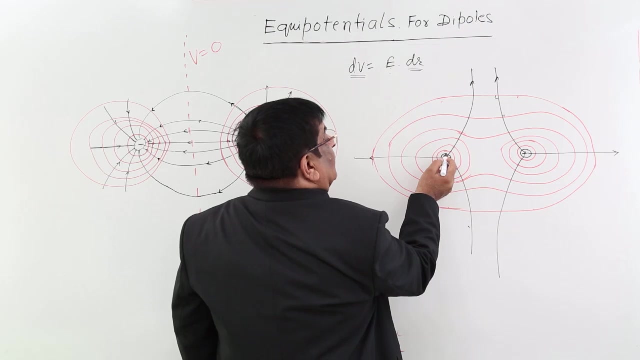 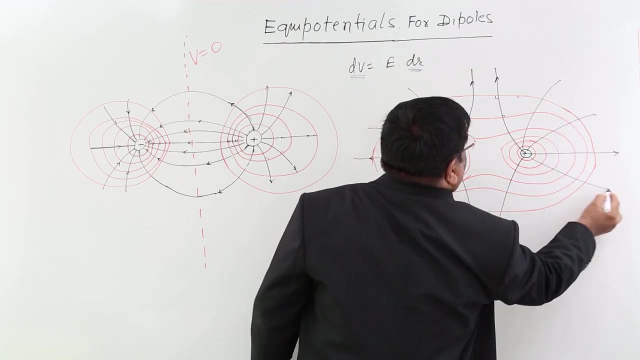 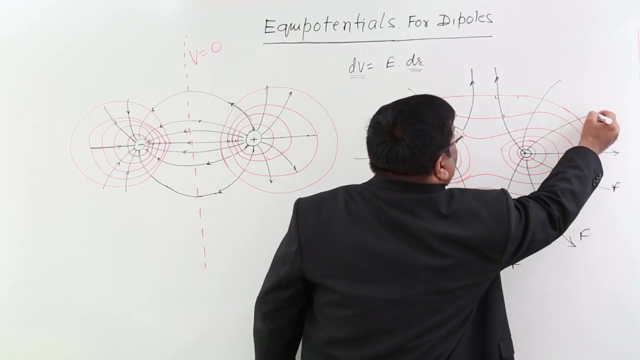 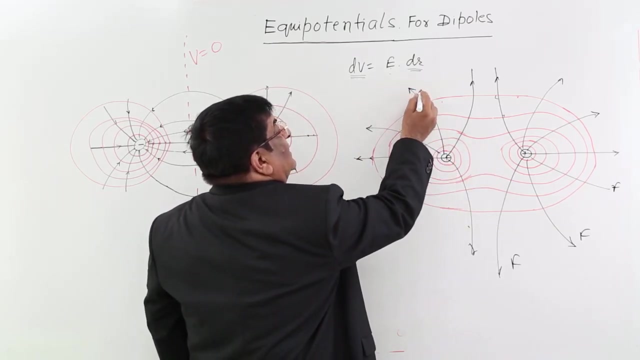 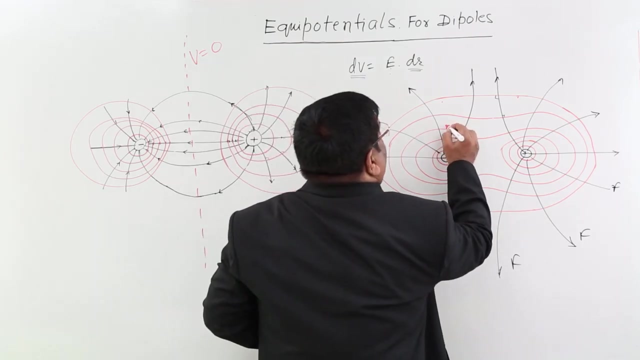 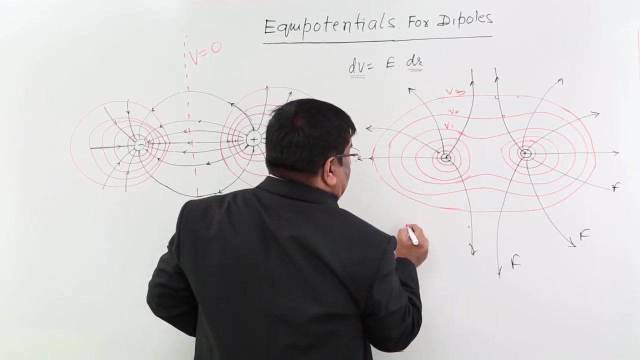 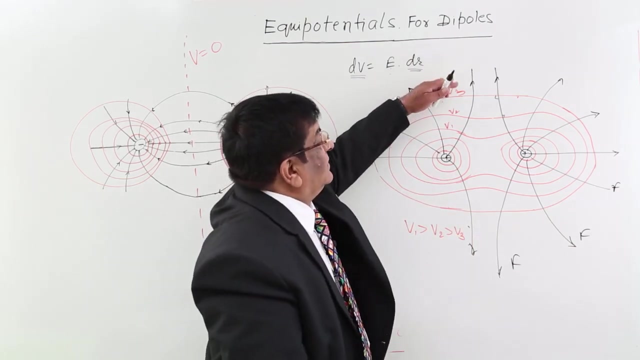 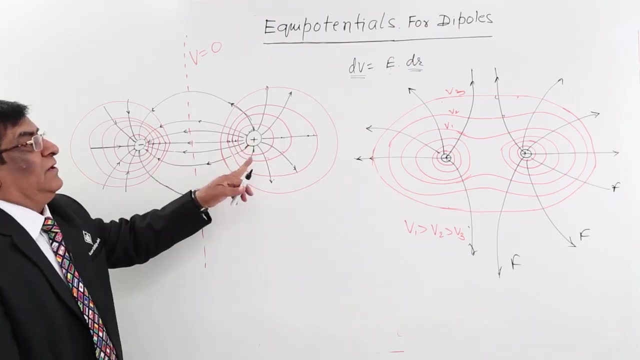 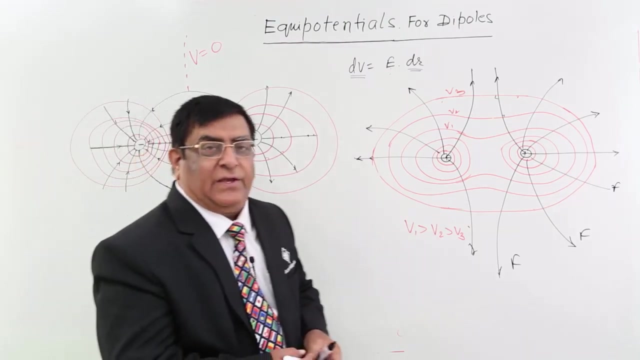 be like this: this: then there is a repulsion between the two. this will be this way. this will be this way.